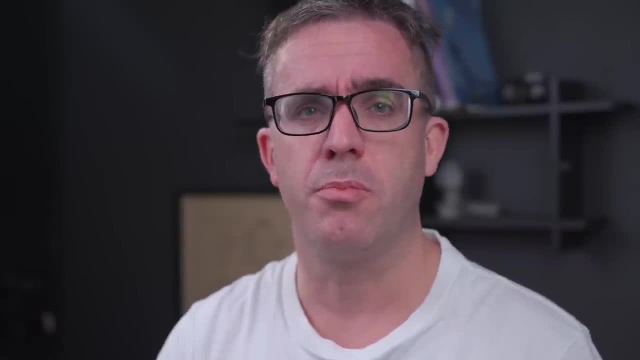 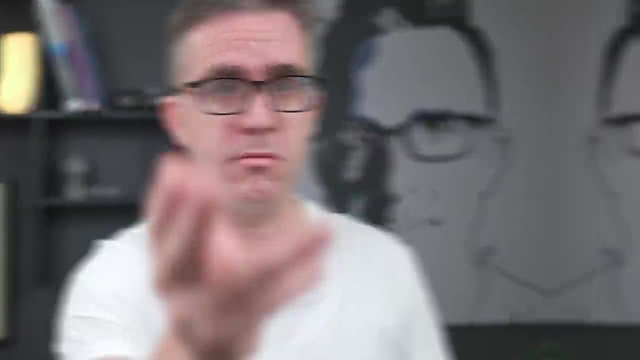 So we're going through the differences. And what is the same about these two professions? In reality, they work on very different areas. My name's Brendan, your structural engineer. Now let's get into it. Both of these professions have really good career path and arcs as they're. 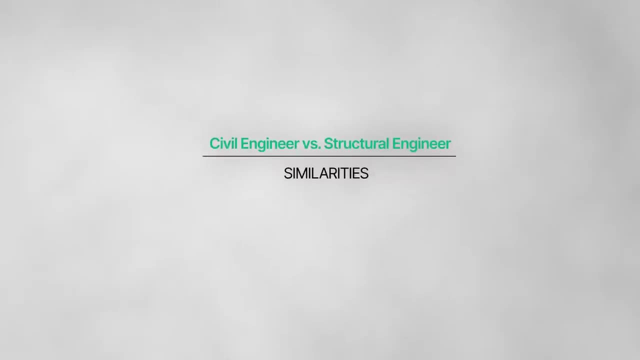 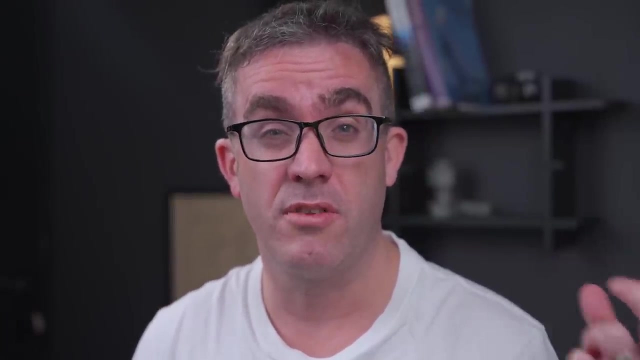 really enjoyable and they work in very similar sectors And you both need to hold a civil engineering degree. So, whether you're a civil engineer, you'll hold a civil engineering degree, or you're a structural engineer, you still hold a civil engineering degree, but you may have. 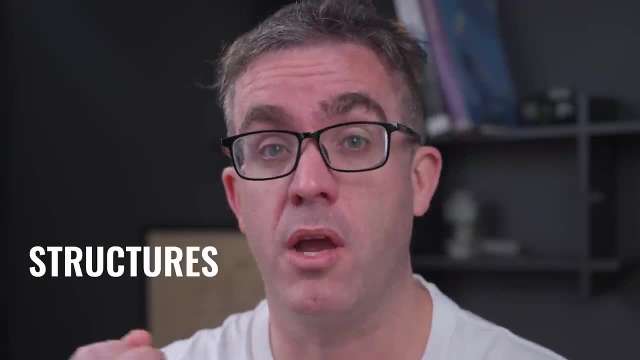 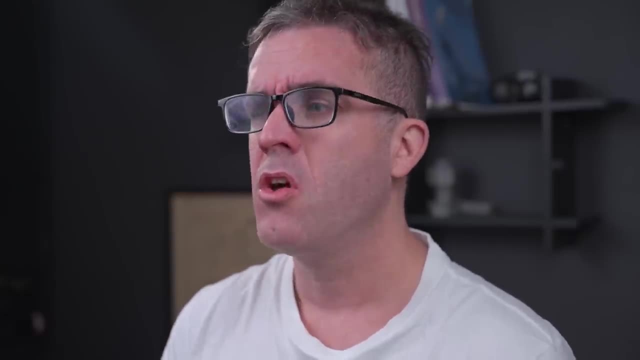 specialized more in structures than the other different sectors that you may have worked on. See, civil engineers and structural engineers have very diverse career paths. It can end up in very different locations working on vastly different projects. So you need to making sure that you're focusing on something that you really enjoy and something 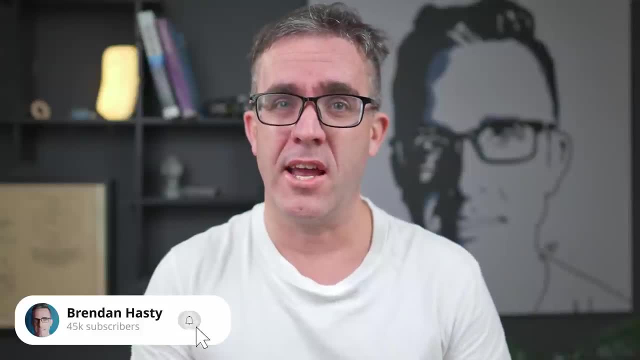 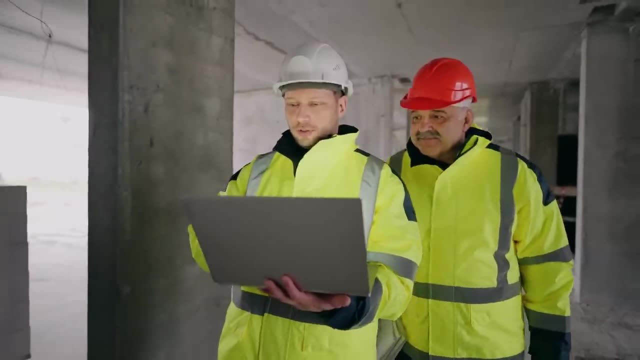 that you want to work on. So where does the similarities lie? As we were starting to say, both of you hold a civil engineering degree At the heart of it, your degree comes from the same area and both will work with the built environment. 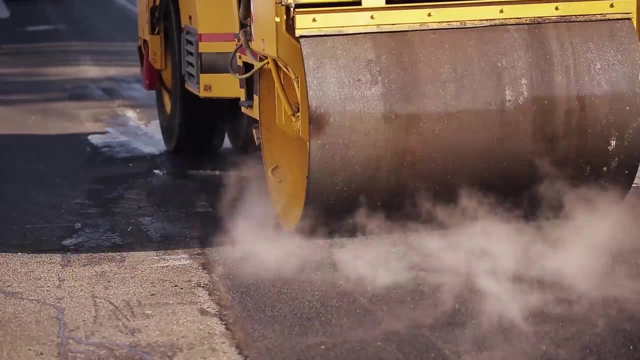 So everything that you can see around you, whether it be houses, infrastructure, roads, drainage, you'll have some sort of interaction with the infrastructure that makes the city tick. So you have the ability to affect many different things, And that's what we're going to talk about in this video. 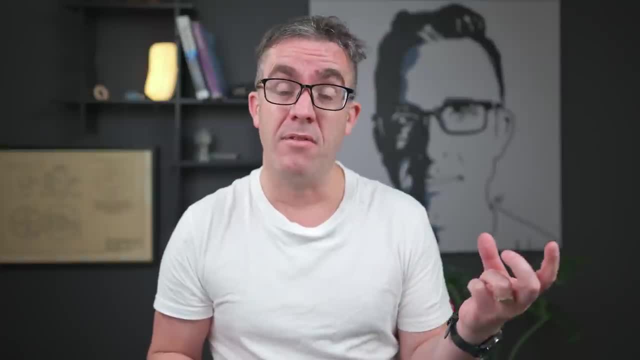 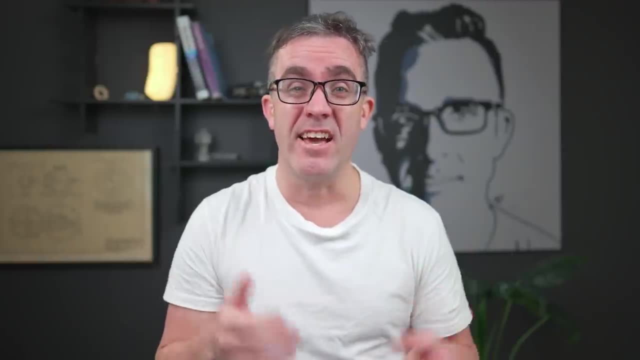 You also both need to have a strong background in maths and physics and how the built environment actually works, as you will be using it day in, day out. It's something that's really required for really any engineer. You can't go past needing those problem solving abilities. 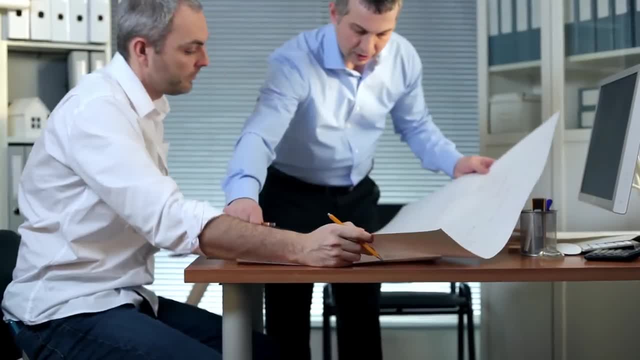 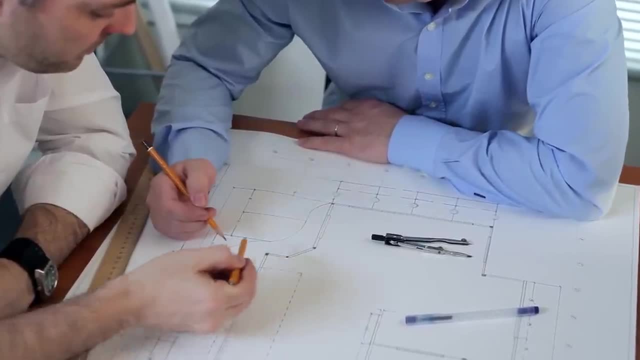 So, whether you're a civil engineer or structural engineer, you need to have a strong problem solving mindset and be able to solve those most complex problems that can see not the most typical results or the most common solutions. Before I go into the differences, I'll break down what actually a structural engineer does and what a civil engineer does. 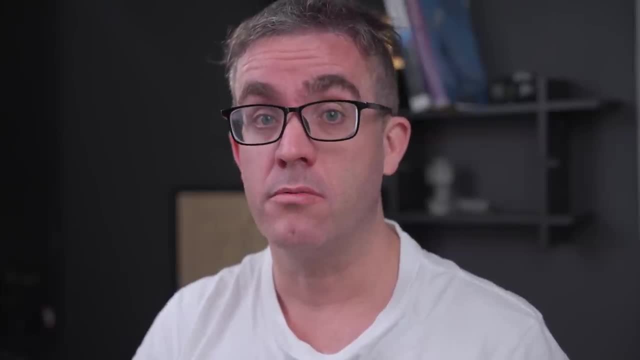 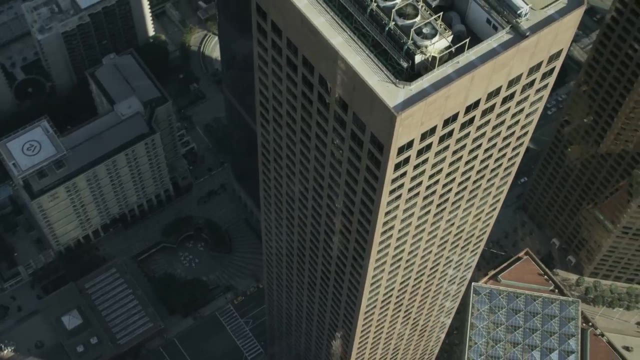 so you can have a better understanding of the type of work you may be working on with both careers. Structural engineer, as the name sounds, you work on structures, whether that be a small residential house, large skyscrapers that change the skyline of any city, or even temporary. 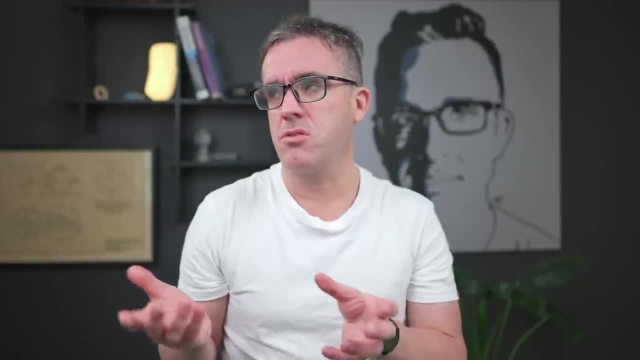 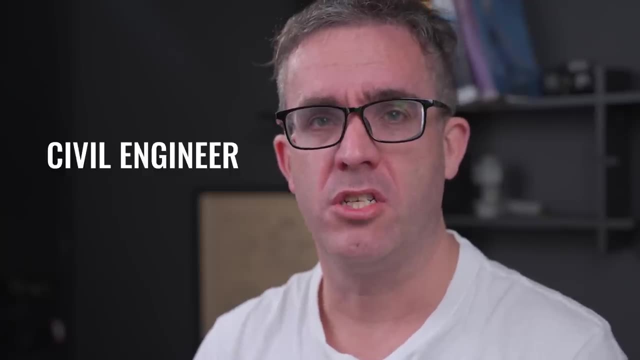 and other structures. This is the type of work that you'd be working on. Even sometimes, structural engineers may be suggested to work on tunnels or bridges, although sometimes that's more related to transport, or even sometimes classed as a civil engineer, as a civil infrastructure. 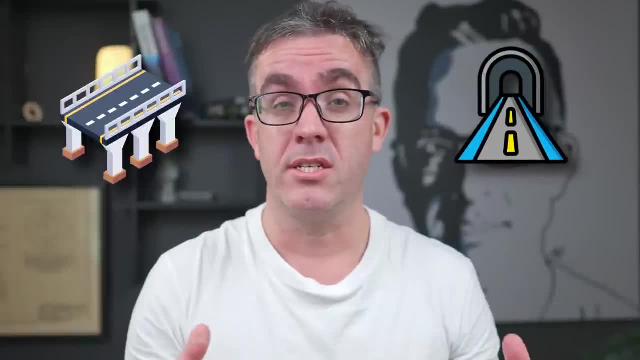 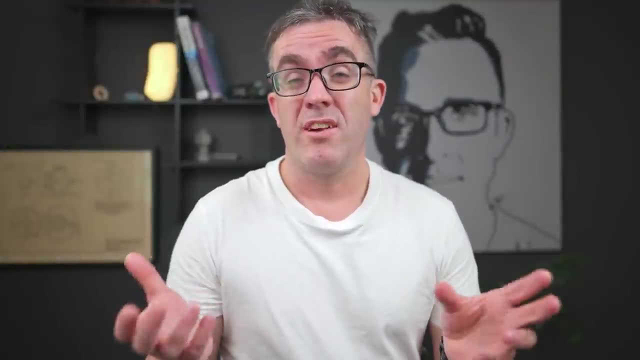 But really at heart, designing things such as tunnels and bridges is structural engineering, as you need to make sure the structure stands up under the loads that are applied to it, So a structural engineer really works on the bones of the structure. When you think about 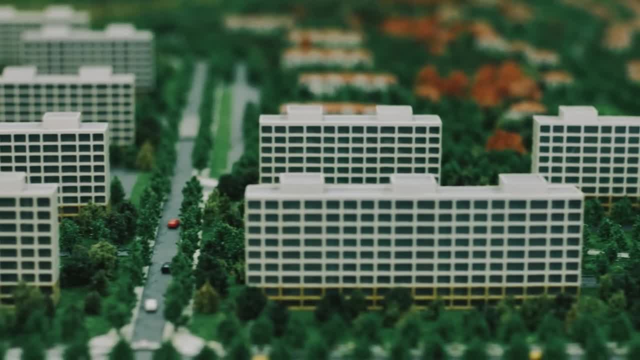 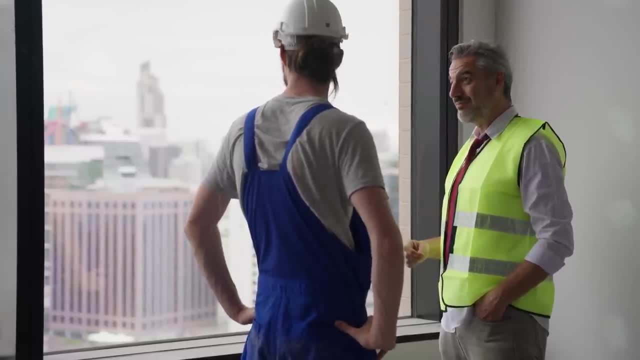 an architect. an architect makes how the building actually looks, flows and interacts with the built environment, While a structural engineer actually makes that dream come into place. So you're making sure that it's structurally sound to resist any loads that may be applied to it. So, whether 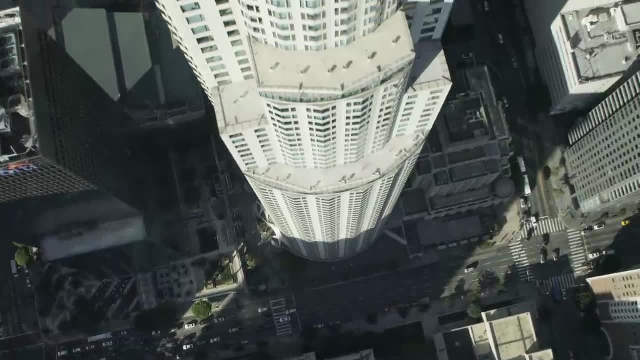 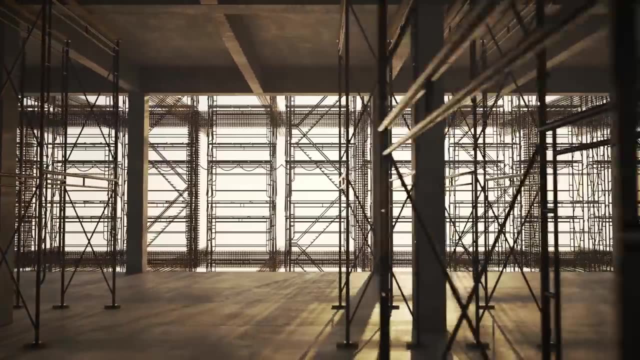 that be lateral loads from wind, making sure that your lateral systems can resist those loads, load from gravity, making sure they're transferring through loads through columns and slabs, and making sure that your ground or floor doesn't vibrate enough to cause impact to the occupants, with 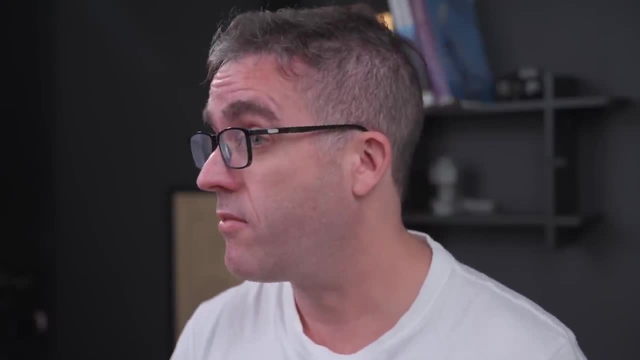 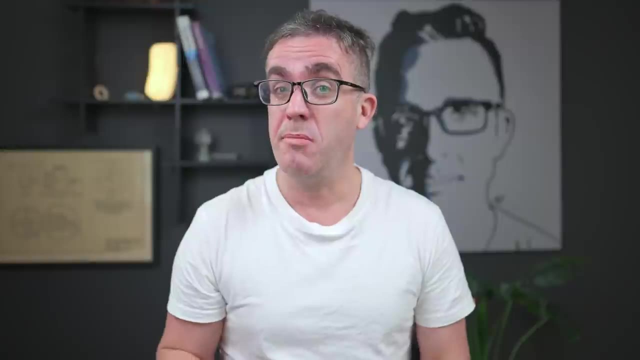 inside, as you can build a structure that is structurally safe but potentially bounces a lot when people are sitting on the floors. now, we've all been in buildings like that and we can see how discomforting it is, so you're making sure that when we are designing them, we are considering 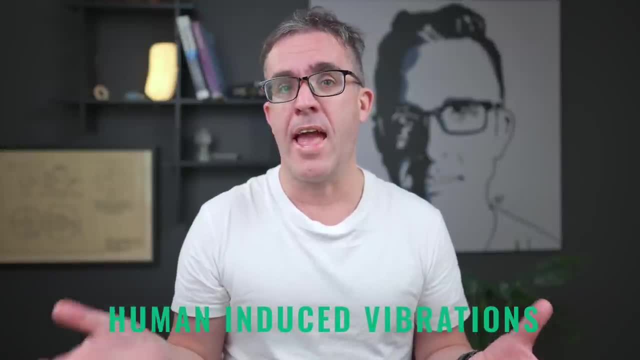 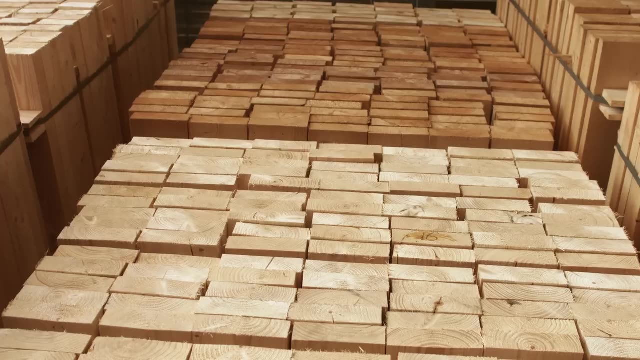 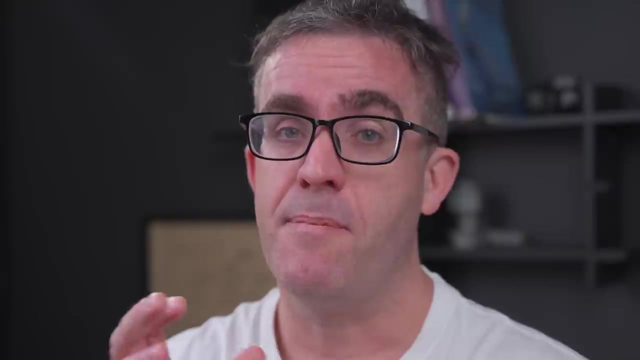 those other aspects of human induced vibration and how it may infect the occupants within. as a structural engineer, you will be working with also different materials, whether it be wood, steel, concrete and even composite materials at some aspects. so you're working with a lot of varying materials and making sure that they're safe and sound for the loads that are applied to them. 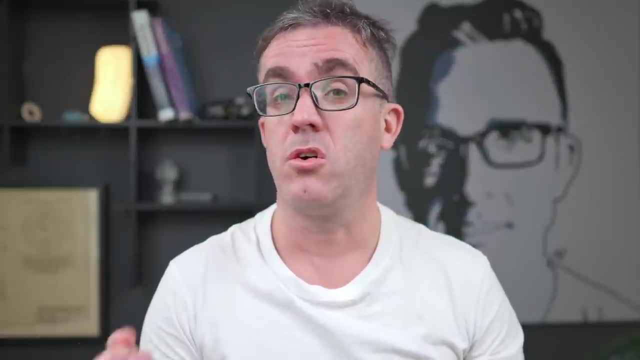 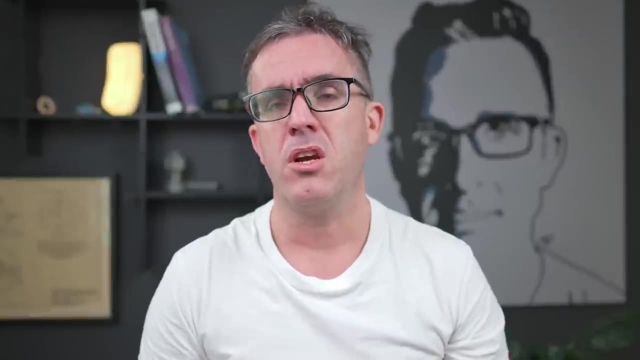 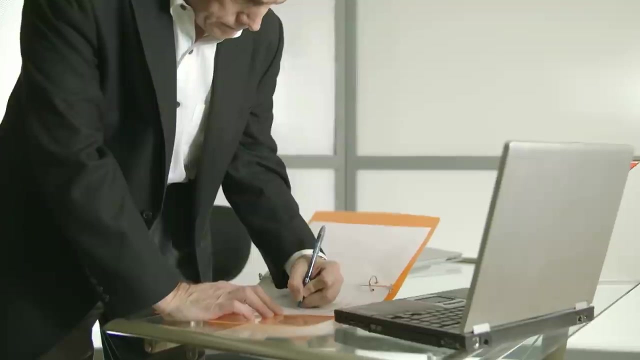 another aspect of structural engineering that people don't often talk about is also assessing the integrity of existing structures or making sure that you're modifying or renovating buildings for different occupancy use. so you'll be going potentially into existing buildings, looking at the structure and evaluating whether it's structurally safe to keep in use and writing reports for any remedial work or repair. 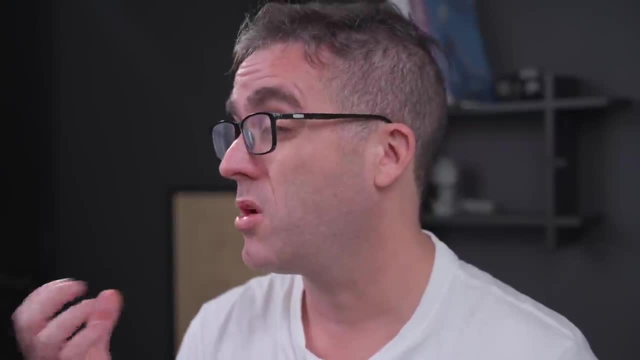 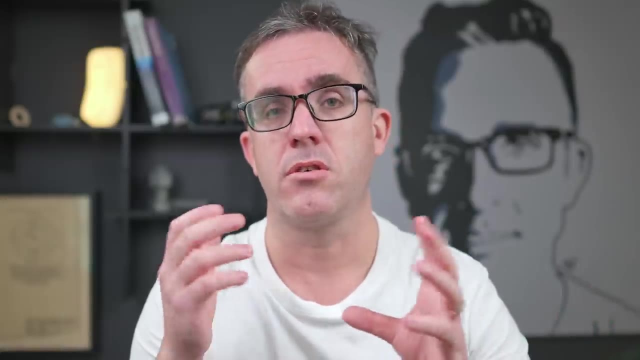 work. Now, repair work is something that people don't think about, but it's really one of the most enjoyable areas that you can work on, as it makes you fully understand how structural engineering works and how this load transfers through a structure. So if you are looking for a structural 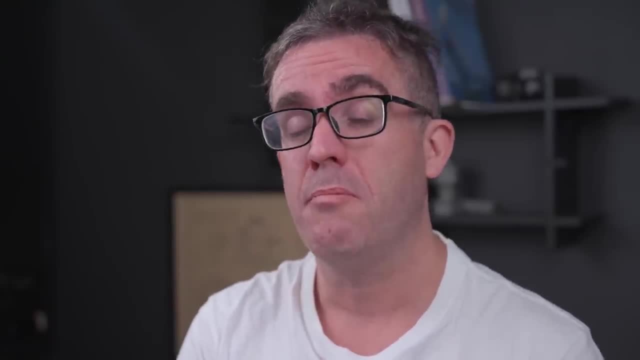 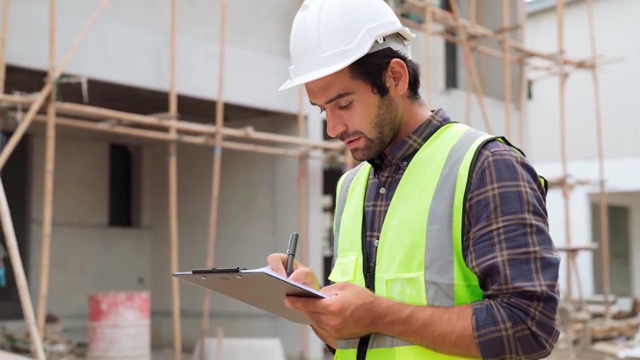 integrity. it's not something that I would necessarily recommend you start off with, but maybe something you look into the future, as you can build those strong design aspects and how buildings actually work, then using it to assess the structural integrity and how you can repair structures and remediate them to make sure they're safe. In short, basically you're. 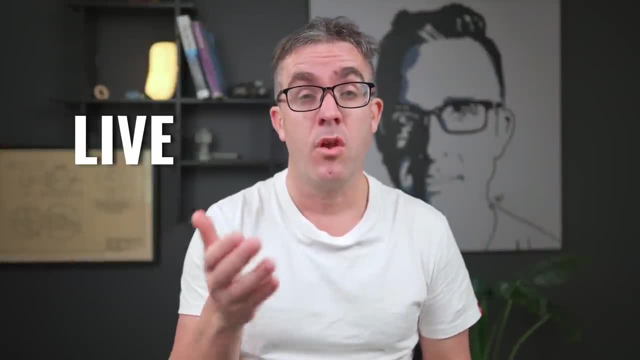 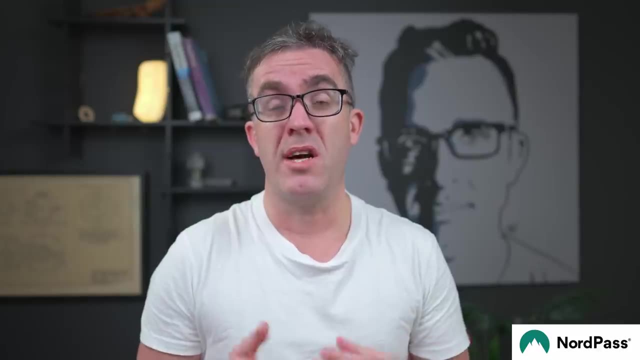 making sure the built environment is safe to live, work and play in, building the bones that the buildings stand up on. This video is sponsored by NordPass. So what is NordPass? NordPass is a password management system for businesses. It allows you to share your most secure data. 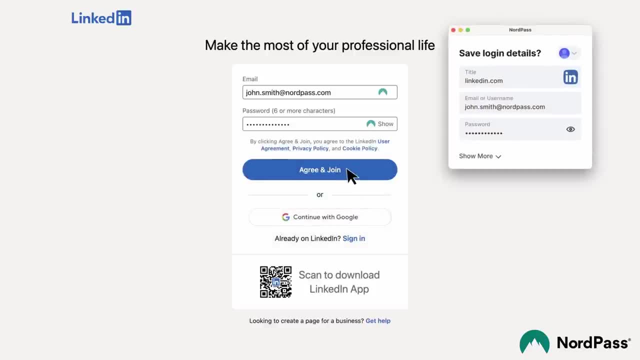 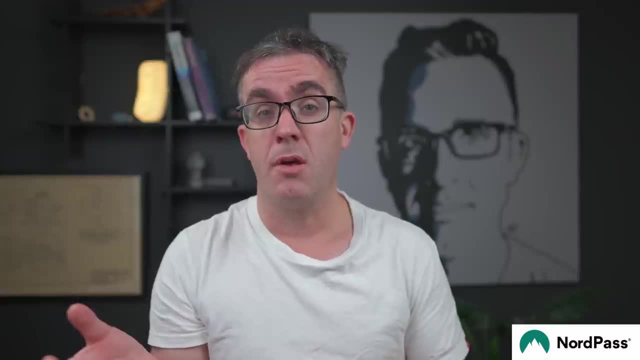 whether it be passwords or payment information. with the highest cybersecurity protocols today, Password management and making sure that your staff is using the most secure passwords at hand can be really helpful. It's really time consuming for all staff, So if you're having to log into things quite regularly, 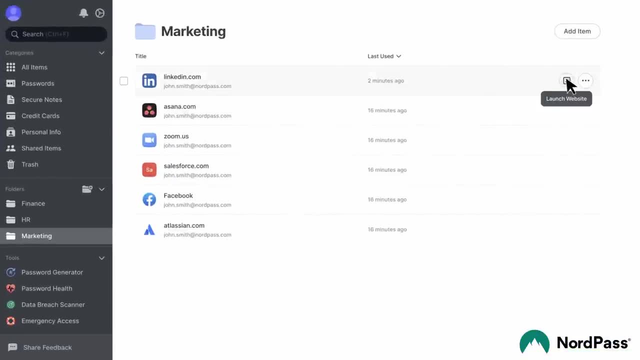 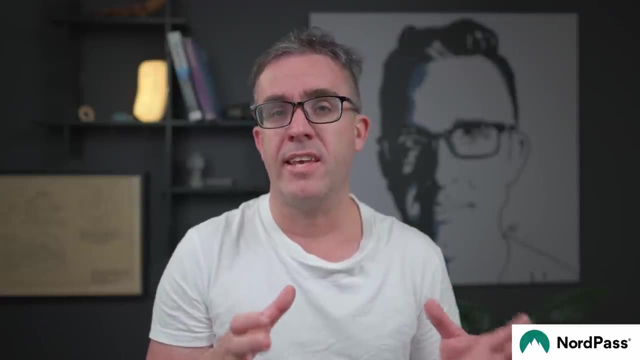 it's quite hard to remember the more complex passwords, meaning that your data is more secure, And NordPass takes this off your hands. with this secure system, It allows you to share that most secure data efficiently, easily and even revoke access quickly, at the touch of your fingertips. 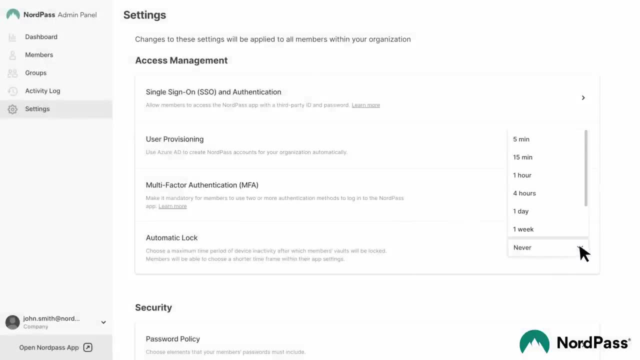 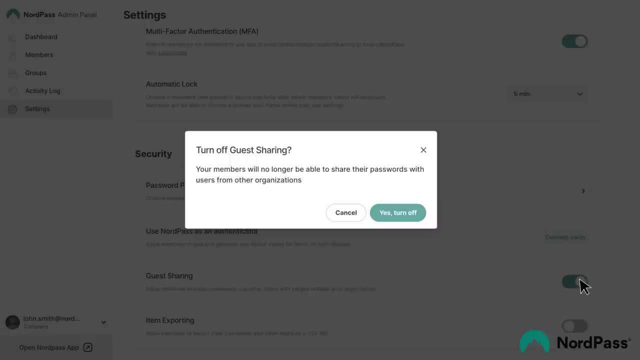 So it means your most important data, which is your password and payment information, is easily controlled and you can control who has access to it by easily revoking access when you need to. As it is primarily also a password based manager, it means that you can quickly scan all the passwords that are being used within your 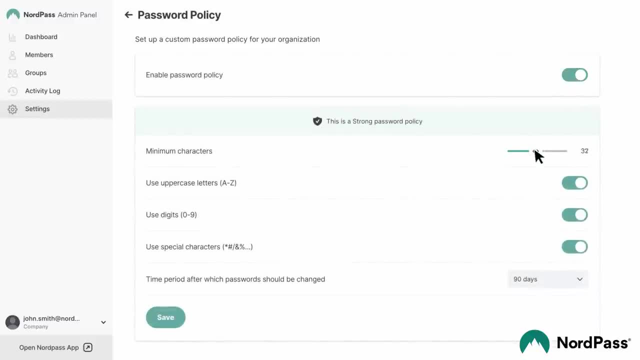 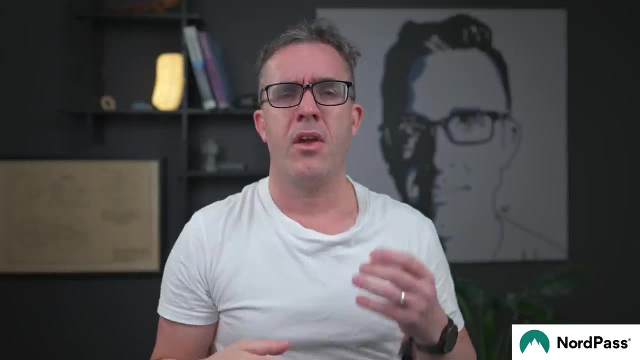 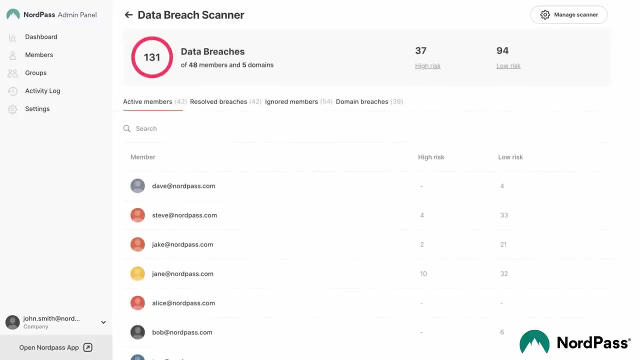 organization, making sure they're the most secure and no repeat or weak passwords, So you can take action wherever you need to to making sure that you're increasing the security of the passwords that you have out there. They also have a data breach scanning system, So it means they scan whenever your data has been leaked. So whenever that occurs, you can quickly jump on top of it, making sure that the damage is at the minimal point possible. 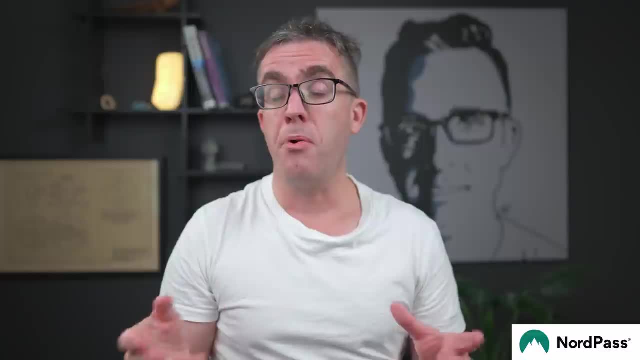 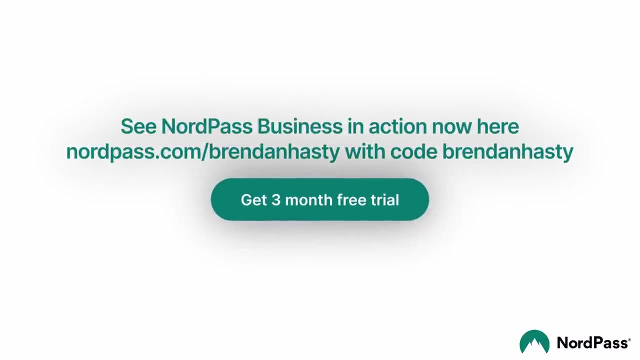 And you might even be able to pick it up Before any damage actually occurs. NordPass is offering a three month free trial to businesses, with the link in the description and using the following code, which means that you can try it risk free and see how it goes and see where that actually suits you and your operation. 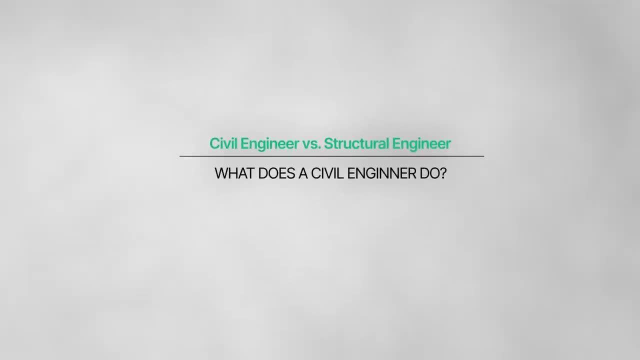 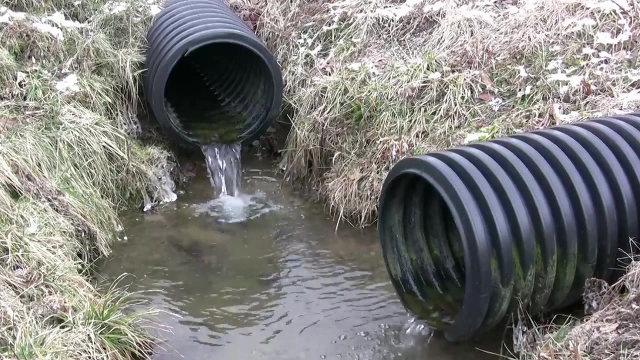 Now let's get back to the content. Let's come into civil engineering. Civil engineering is slightly different. Typically, you're interacting with how the actual planning and drainage of this interface works. So potentially you're looking at either a single building and how the drainage comes down out to the outlet. 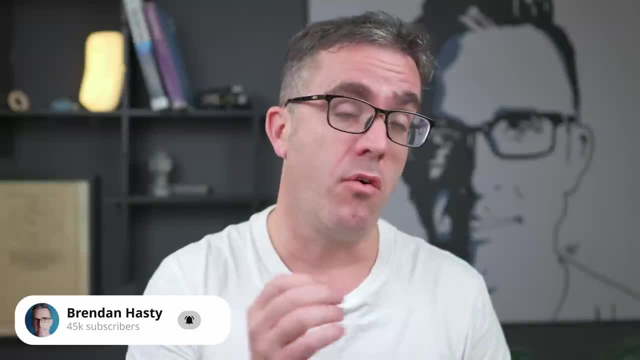 So you're looking at big developments of how the overland flow goes, making sure that you're not flooding any specific location where the flow may go through, making sure that it's got a path through it, so don't flood out specific structures. 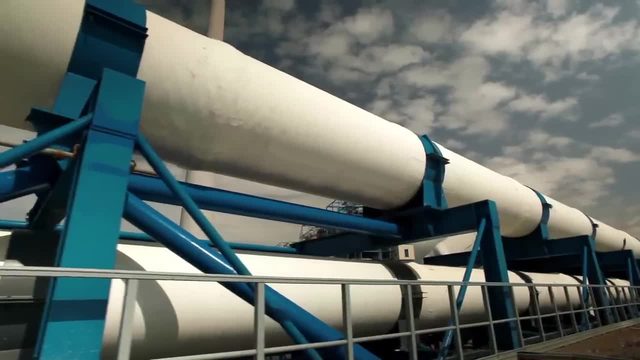 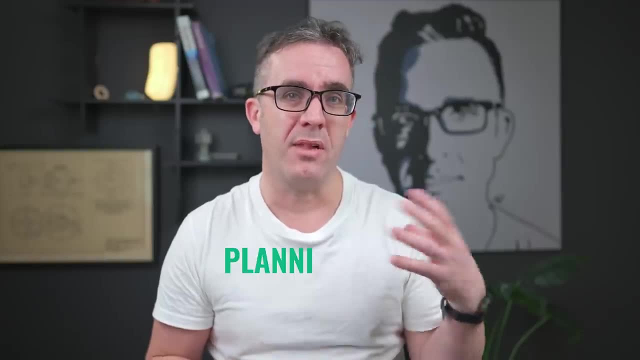 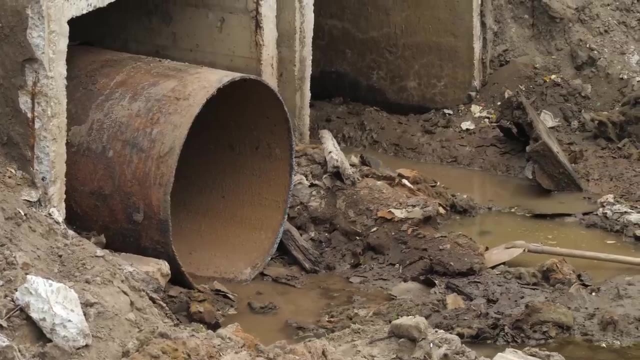 You'd also be looking at where roads go, how they're shaped and where the drainage comes from, So you're making sure that there is correct flow and pathing through certain developments. So, whether it be those planning, developments or drainage systems, and something that is not often thought about is how the drainage systems actually work, as they're really invisible, they're hidden below ground and work. 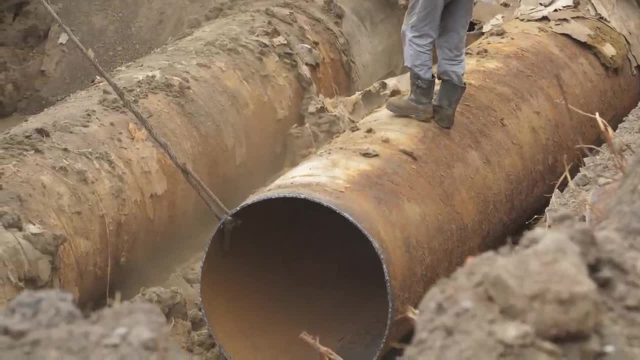 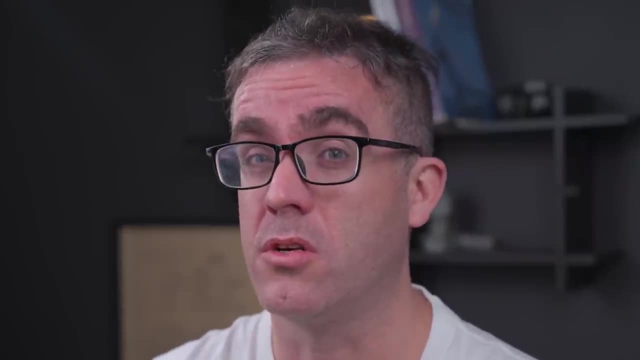 Where things don't work. you quite often see it in a lot of floods and other environments, So the only time that it comes into play is when the drainage system doesn't actually work, as they're quite invisible and something that's quite often overlooked but is extremely important for a functioning society. 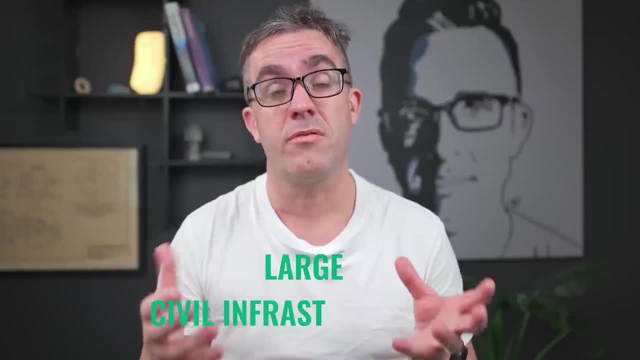 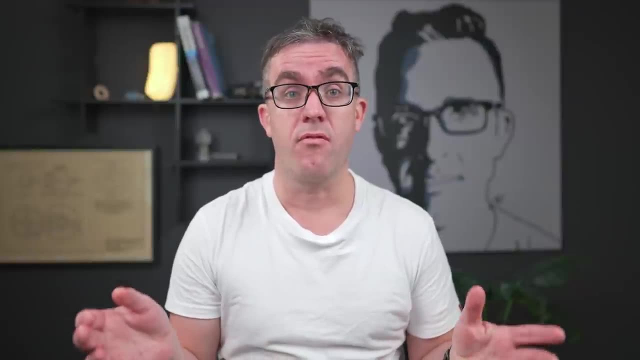 Other areas that you may be looking at is such things as large civil infrastructure, whether that be large retaining walls, culverts or other aspects like that, So where you're shaping the ground and the environment around it, making sure that it's functional for what it needs to be useful, making sure that you're not, either, getting flooding. or roads that are too steep- meaning the car bottoms out- or corners that are too sharp for the speeds that are applied to them. Well, sometimes it doesn't always work out, as in hilly and windy structures. Sometimes you just need to have those curves, but you will potentially set the speed limits on those corners. 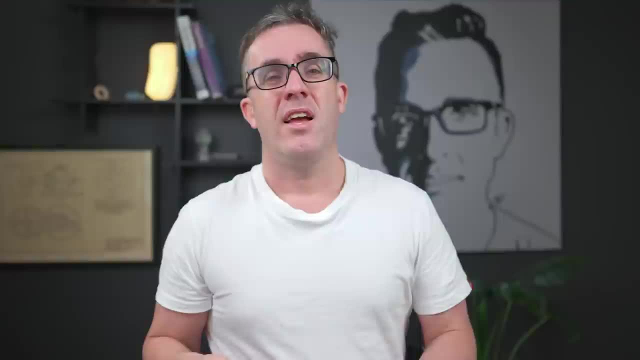 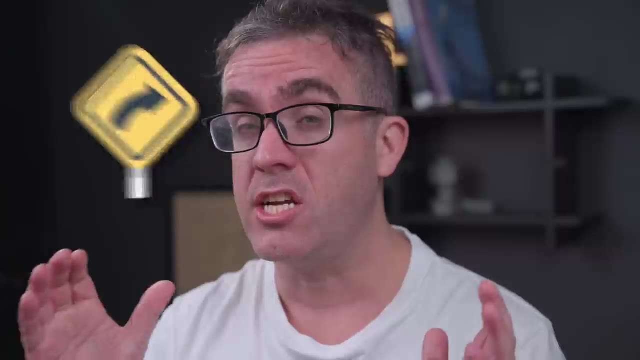 As you can see, those yellow signs for the suggested speed limit around those corners. As sometimes in hilly and windy environments, you don't have control over how sharp those corners are going to be, So that's where you get those suggested speed signs saying that this is how fast this corner has been designed for for optimal use. 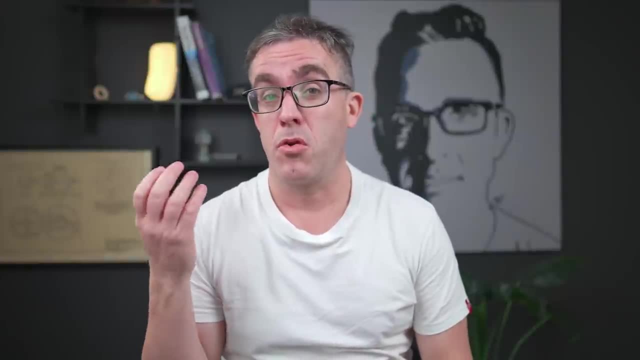 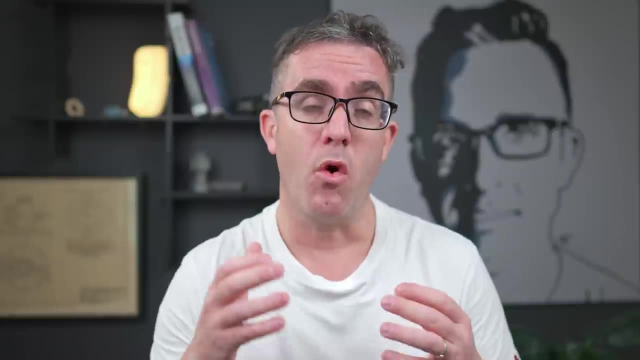 to make a sure that it's safe. Civil engineering can also sometimes be thought about working on bigger infrastructure works, So whether it be your big bridges, tunnels or other environments like that, So it's really working with the soil and shaping it to making sure that it both has access and drainage for what it needs to be. 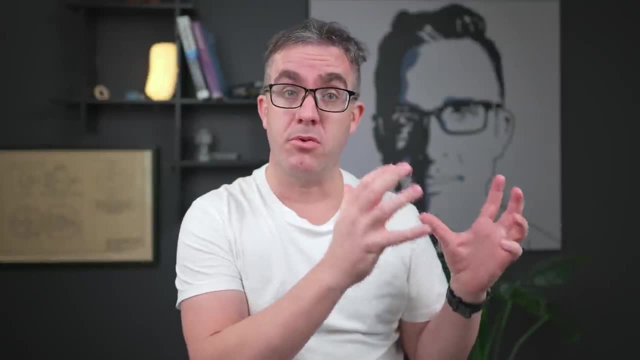 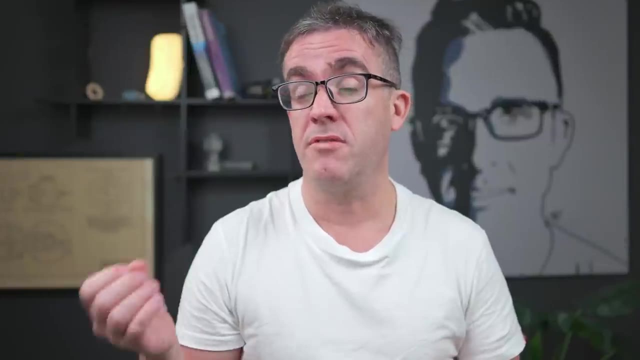 But a lot of time. those bigger aspects normally get lumped in the transport sector. So you might be a civil engineer in the transport sector working on those type of projects. So whether you're in the profession, quite often a civil engineer, you're normally working with the drainage, planning and 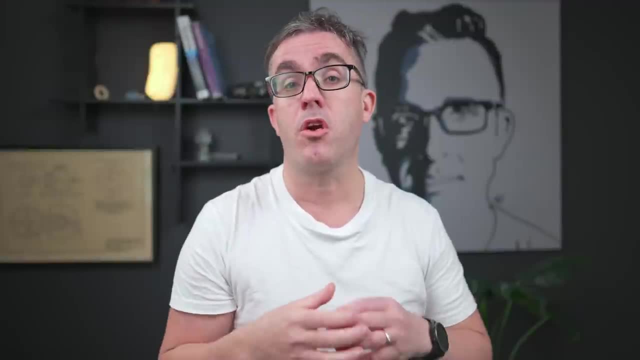 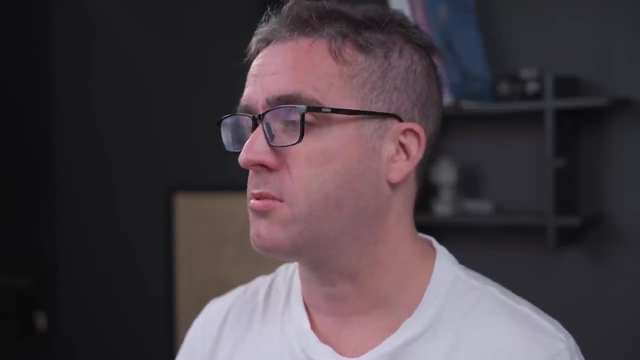 other aspects like that, Where a civil engineer in the transport sector will be working on that more bigger infrastructure, like large infrastructure systems, like big retaining walls, big bridges, tunnels and other aspects like that. So there's a slight variation depending on whether you're in the civil sector or the public sector, depending on what you're working on. 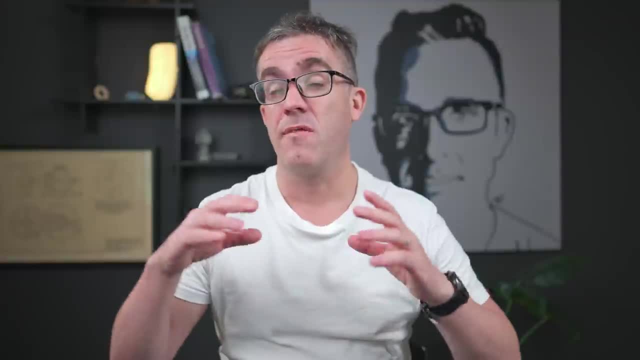 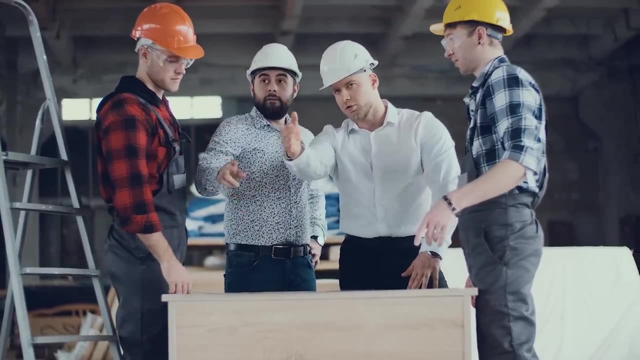 But, as we can see, the problem is civil engineering is kind of like a broader topic, So depending on what business you're working on, your work can vary greatly. So there's a big variety of work that you can potentially work on Where in structures it's quite easy.